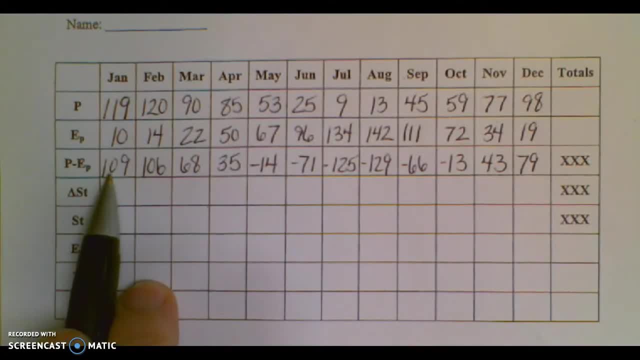 look at January, you'll see that, even if it was zero the month before in December, there's more than enough rainfall in this month to overcome potential evaporation and get your storage back up to 100.. Same thing for February. It's not always going to be that way, though You're not. 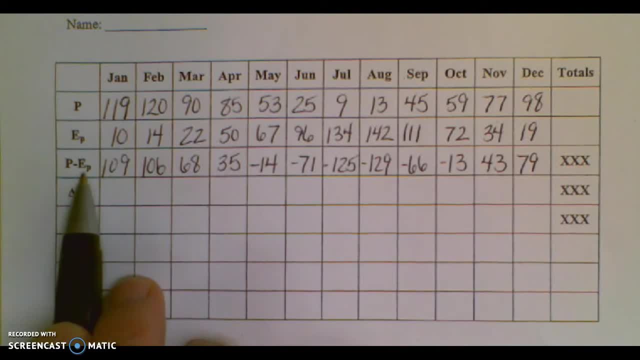 always going to have a P that is greater than 100 over your E sub P. So looking at some of these numbers here, you'll see that you know 68,, 35, that's more common to what you're going to be. 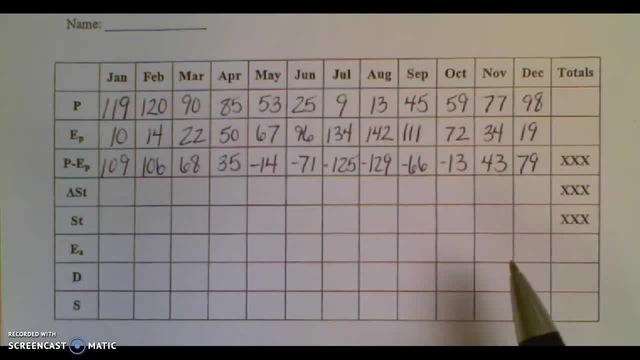 seeing, You can also go and take a look at your areas of the year where your storage might be zero. So, worst or best case scenario, however you want to look at it, May, if it's 100 the month before, if your storage is 100 the month before, it's going to be down here, it's going to be a 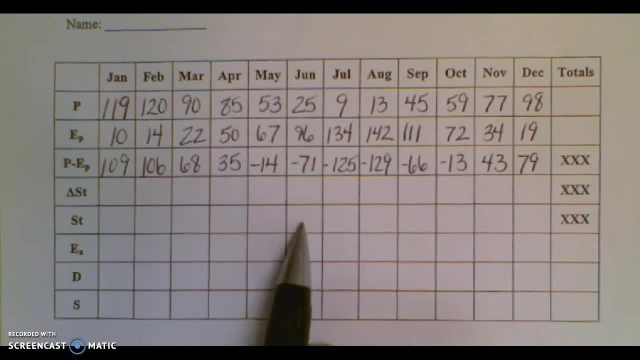 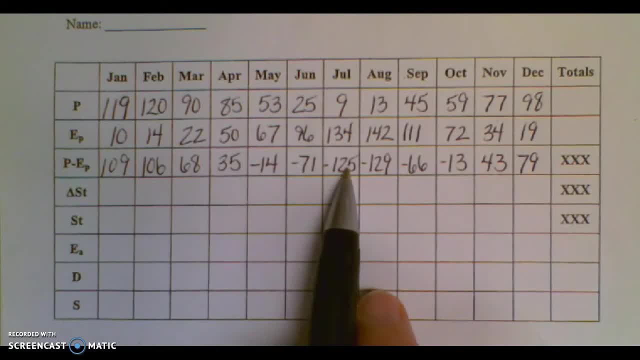 that even if my storage was 100 in April, I would definitely be down to zero. So I could put a zero here for storage for July and know that that would be my starting point. so I could start in August Or I could go back up here to January and February and work it out there, But I already had the zero. 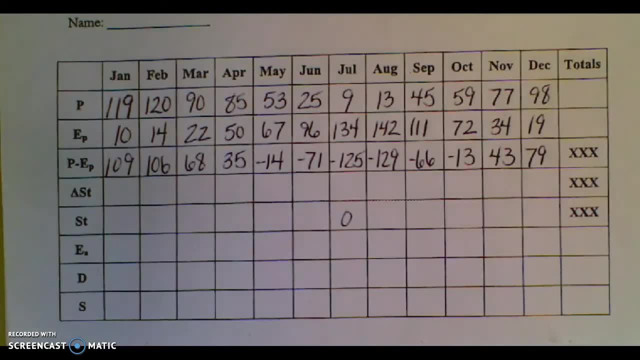 on here. so let me start in July. So there's two ways you can do it. You can go through and work vertically, filling in each column month by month, by month. or you could work horizontally and fill in the row, fill in all your storage and your change in storage, fill in all your actual 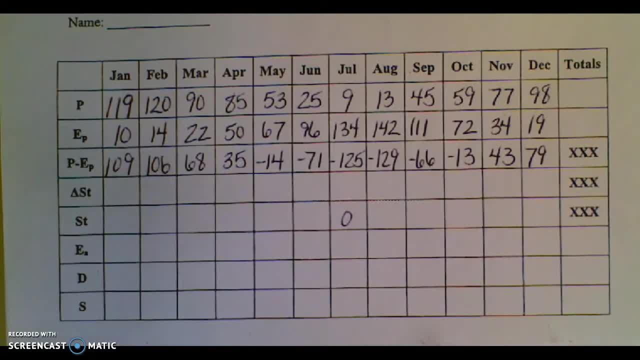 evaporation. whichever you prefer, Once you get comfortable with it. usually it's better to go horizontally. You can go a little bit faster, but you know your preference. I'll do it both ways so you can see how it works, And I'll start out by going vertically through a column. So July is my. 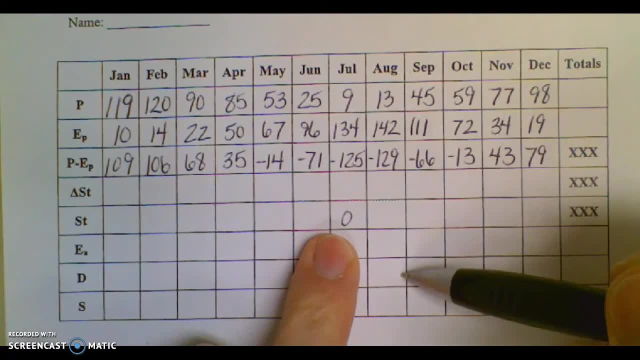 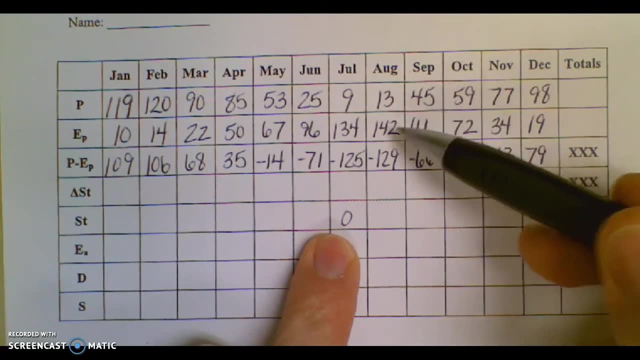 starting point, which means I'm really filling in August. first Notice for the month of August: it's dry. I'm getting 13 millimeters of rainfall from the sky, but I want to evaporate 142.. Okay, chances are. this is a. 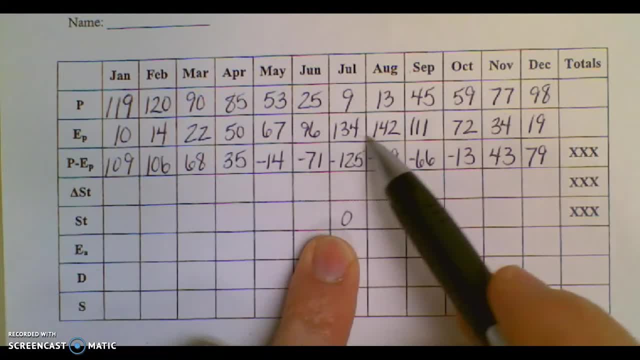 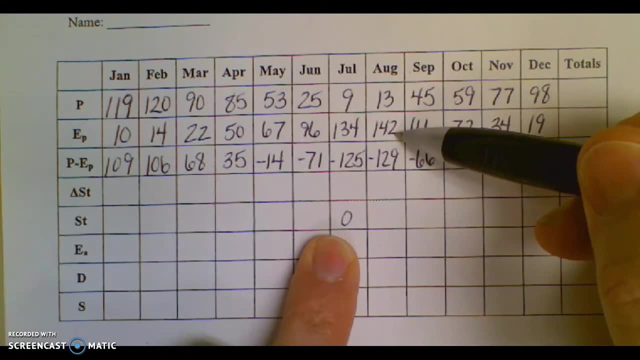 northern hemisphere city. Notice how the potential evaporation increases during the summer months, decreases in the colder season. A lot more evaporation occurring on the ground, a lot more leaves in the trees. So you can see I'm short. 129 millimeters of water. Now where do you go to get? 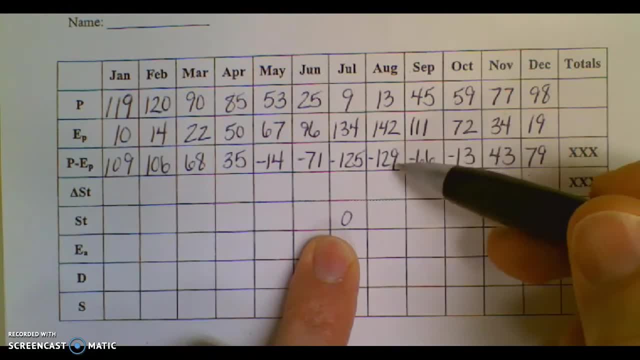 that extra water. Well, in most of the months you're going to go into storage and get it. But notice the previous month. We don't have anything. So if we already don't have anything in storage, then we're going to stay at 0, which 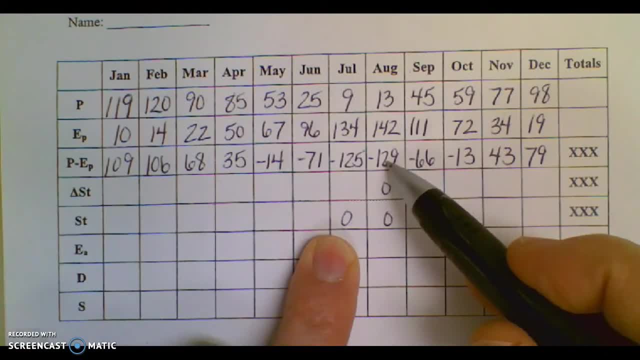 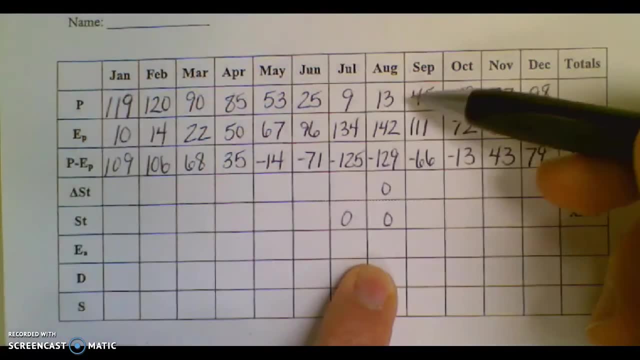 means the change is 0.. I'm trying to take 129 millimeters of water out of something that doesn't have any water. So what's my actual evaporation that month? Well, how much water did I have to work with? Just because I didn't have any on the ground doesn't mean I didn't have any water. I. 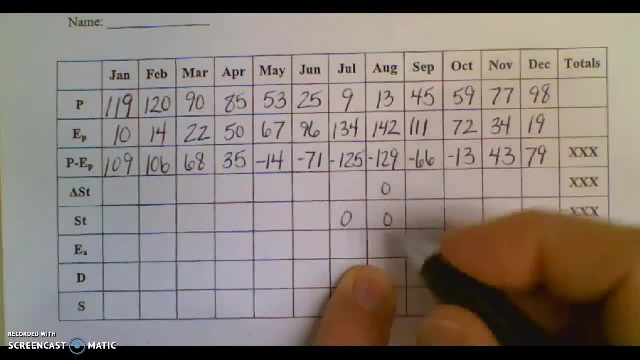 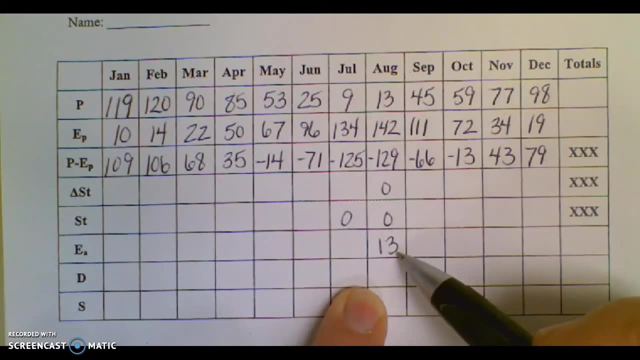 still had 13 millimeters fall from the sky. So that's what evaporated: 13 millimeters that came from the sky. guy, Am I running a deficit? You bet I'm running a deficit this month. I wanted to evaporate 129.. 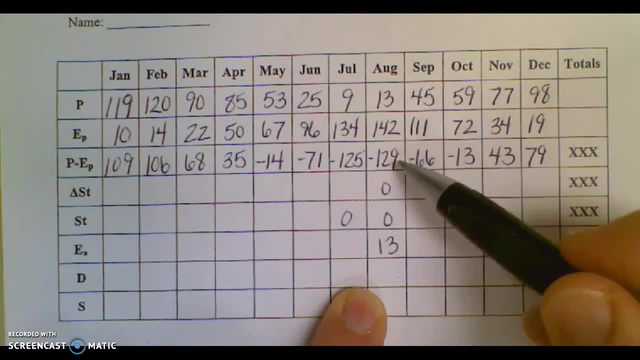 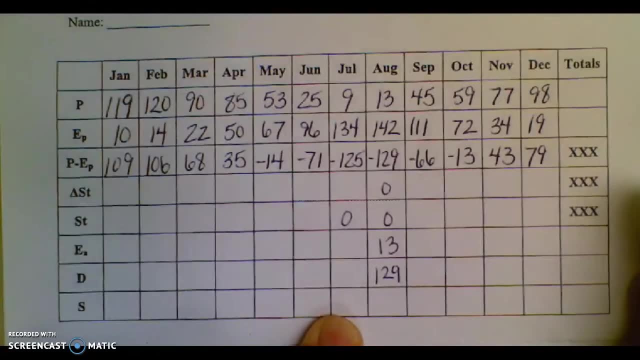 I'm sorry. I wanted to evaporate 142, but I was 129 short, So that's my deficit. And obviously if you have a deficit you can't have a surplus, So my surplus is zero. Moving on to September, you'd do it very similarly. It's another dry. 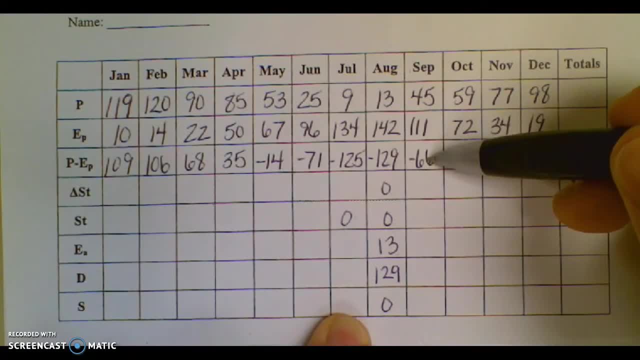 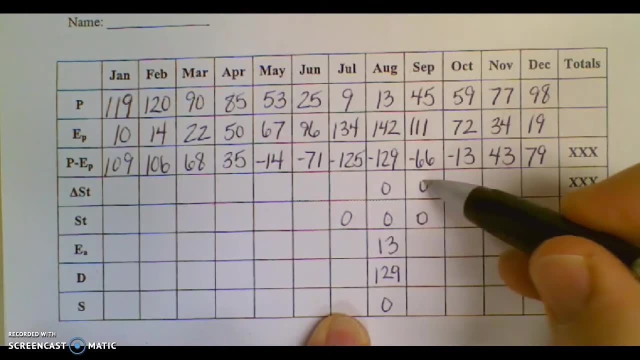 month I'm still looking for 66 millimeters of water. I can't get it out of storage because it's already zero. So that stays zero, which means my change from zero to zero. the change is zero. So zero minus zero is zero. The actual evaporation, since I'm not getting anything. 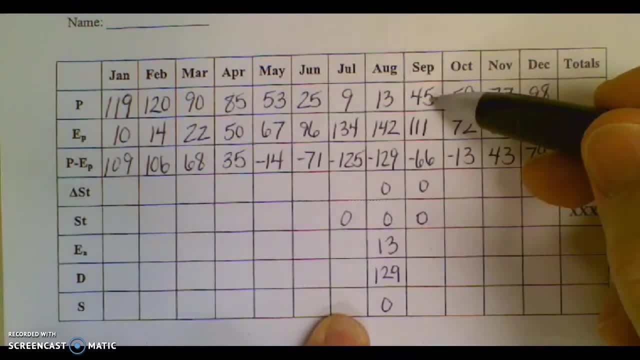 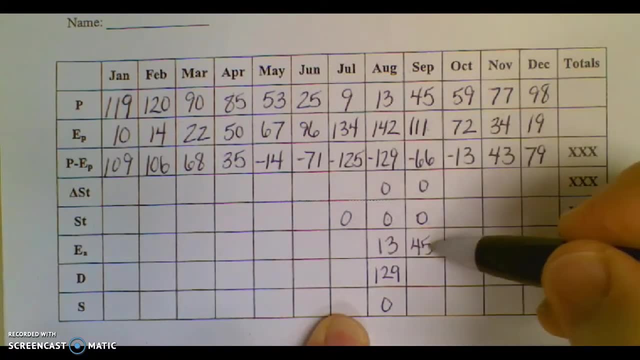 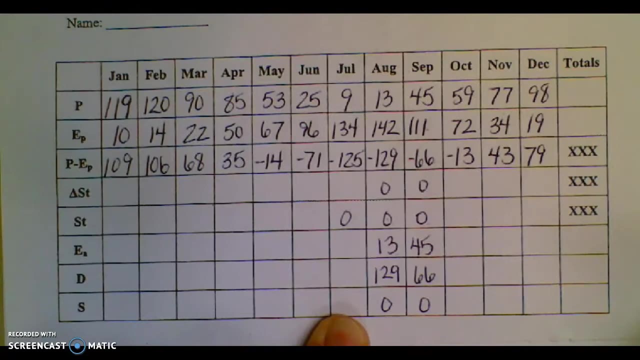 out of the ground. the only evaporation is what falls from the sky, which is 45. And because I wanted to evaporate 111, but I only evaporated 45,, I'm still short, So 66, that's my deficit, And with a deficit you can't have surplus. 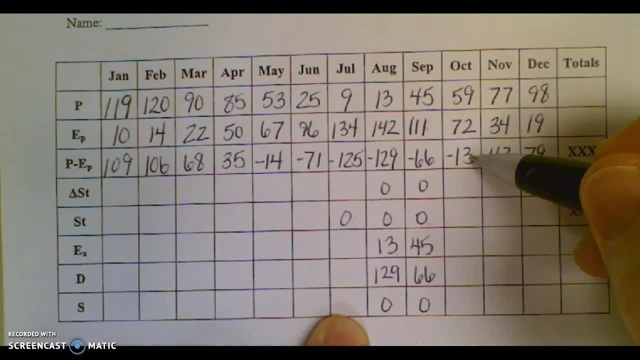 October: again another dry month. Please pause the video now. Try to do October by yourself and then push play to see the answer. So for October: another dry month. I'm looking for 13 millimeters of water. I look to the ground. 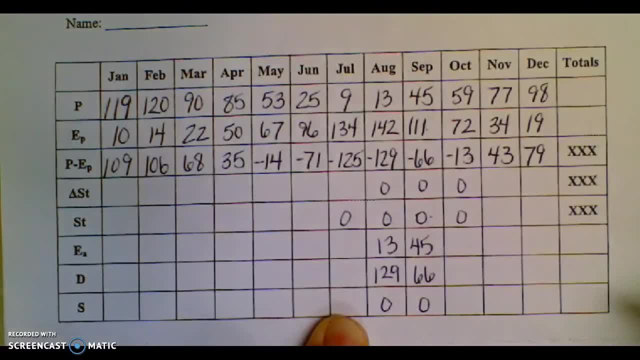 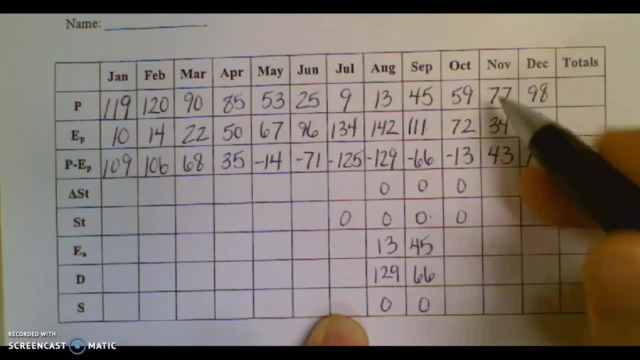 It's not there, So there's zero change, which keeps it at zero. Actual evaporation is just what falls from the sky, because I'm not getting anything out of the ground. So the 59 that fell from the sky is the 59 that I evaporate that month, leaving me still short. I wanted 72.. I only 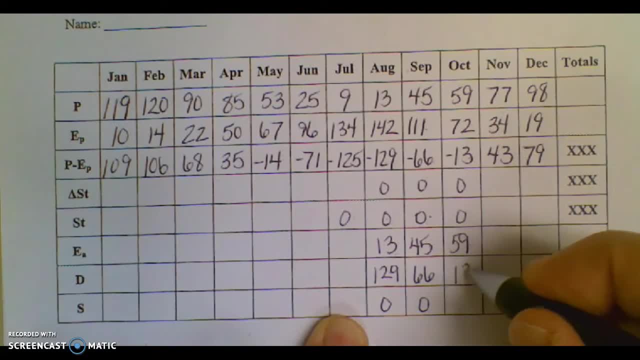 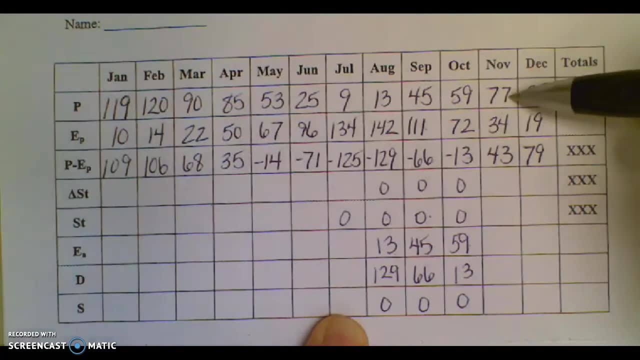 evaporated 59. That means I'm 13 short and I can't have a surplus. Now things change in November. In November I actually have more precipitation, Then evaporation, which means I can start adding this extra water. It looks like I have. 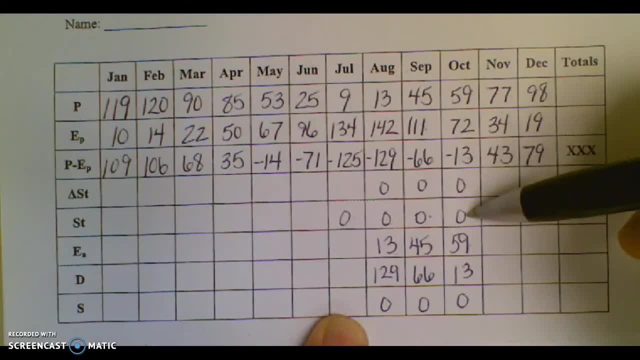 43 millimeters of water. Where is it going to go? It's going to go into storage. I'm going to start recharging my storage, So I add 43, the extra 43 that I had this month. So zero plus 43 gives me a total of 43 in the ground at the end of the month. Now the 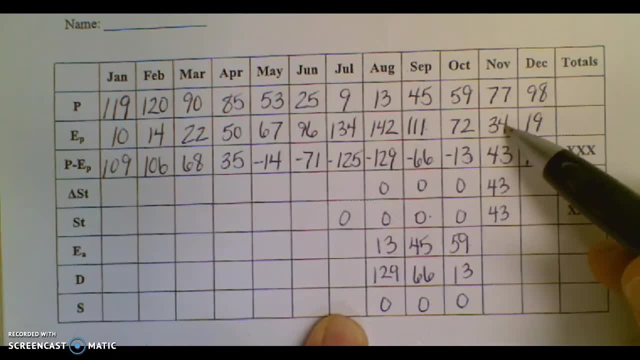 actual evaporation that I wanted was 34.. I had enough water. I had enough water that fell from the sky, So I did what I was supposed to do. My actual and my potential are the same. Am I running a deficit? No, As long as your actual and your potential are the same, you don't have 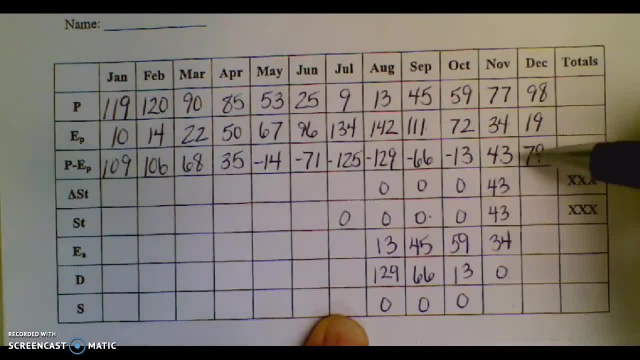 a deficit? Do I have a surplus? Well, some people would say, yeah, I have a surplus because I had an extra 43. But you can't have a surplus until your storage is full. So, even though it looks like I have an extra 43, because those 43 go into the ground, they're soaking. 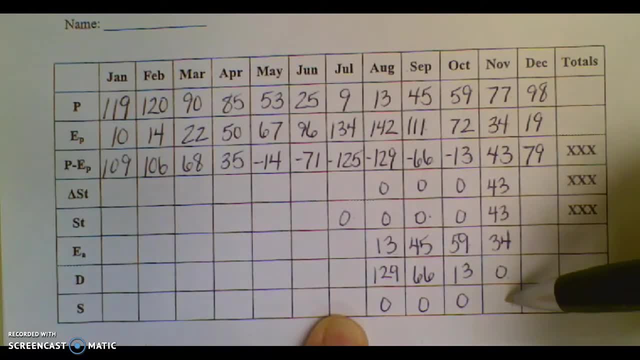 into the ground. I don't have a surplus. Think of a surplus as extra water that can't go into the ground, that has to run off into rivers and streams and then be brought out of the watershed. So still don't have a surplus there. I can't have one until my storage is 100, which looks like it's going to happen. 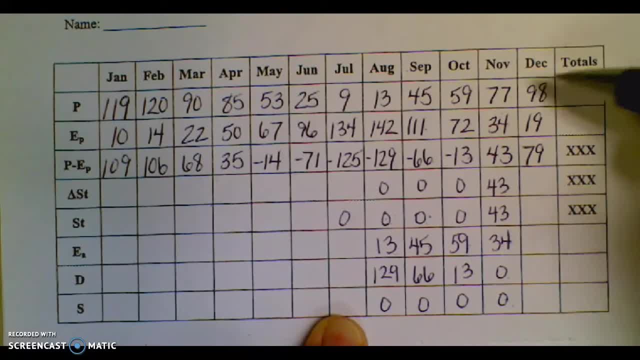 the next month, In December, I've got 98 falling from the sky, 98 millimeters. I'm only trying to evaporate 19.. So now I have an extra 79.. Well, where do you put that 79?? You're going. 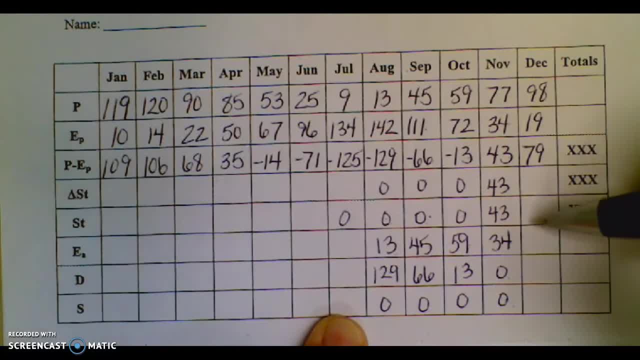 to try to put as much of it as you can in the ground. Remember, storage only maxes out at 100.. You can't put any more than that in. So how much is going to go into storage? It looks like only 57 is going to go into storage, because 43 plus 57 is my 100.. Did our actual 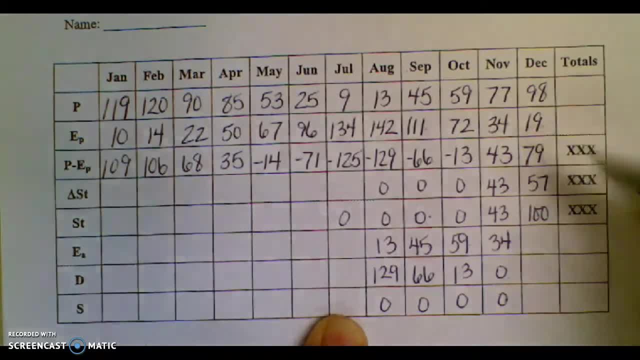 equal our potential. Definitely. I had more than enough water to do that. So those are equal. Am I running a deficit? No, As long as your potential and your actual are the same, we don't have a deficit. And do we have a surplus? In this case, we do. Now, this is a slightly tricky one, because 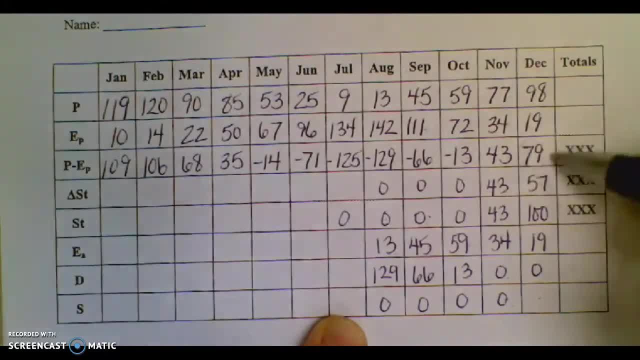 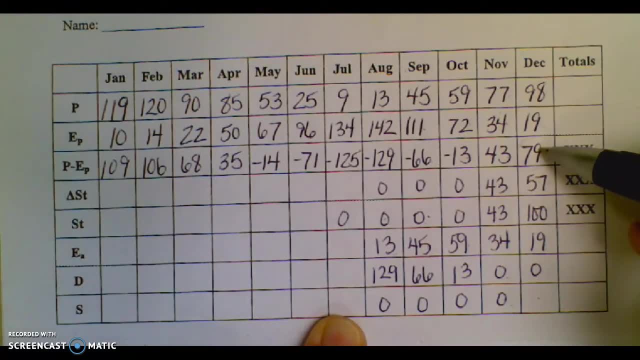 some of this water. okay, I had 79 extra millimeters of water. Some of it actually went into storage, but not all of it. It looks like 22 millimeters, right, 79. Take away the 57. 22 didn't go. 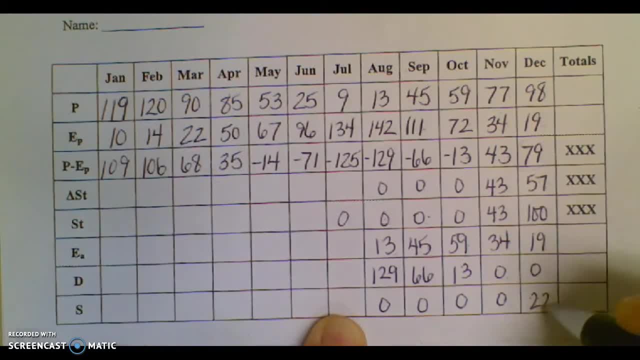 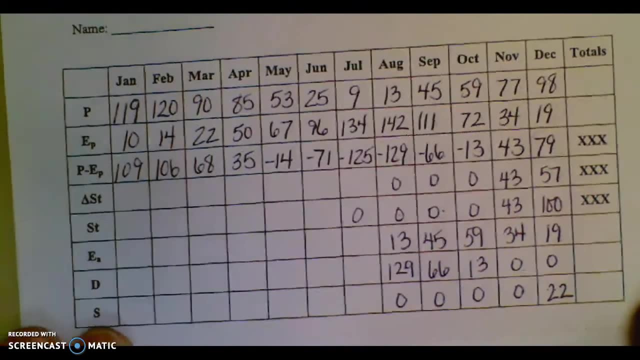 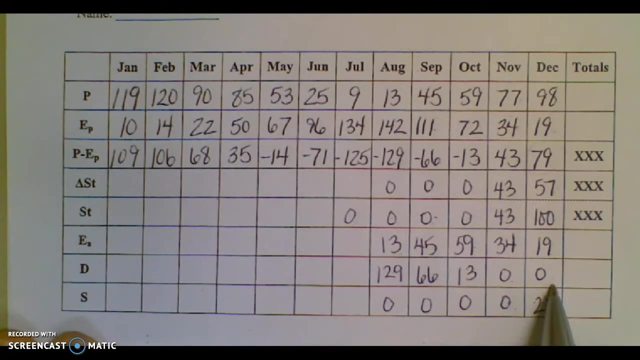 into the ground. So the 22 is what I had. So I have enough left over for December. Moving on to January, I'll do one more month vertically before I go horizontal. January is the month that follows December, so I'm going to have to use some of this information. 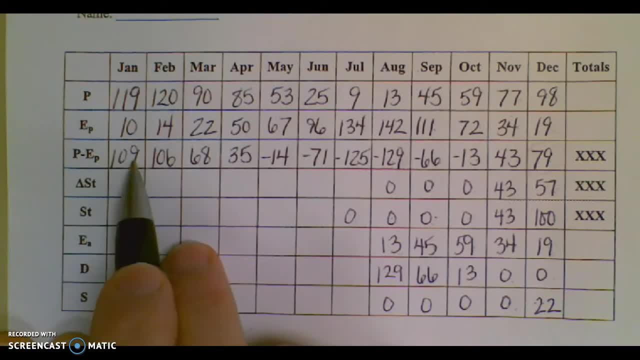 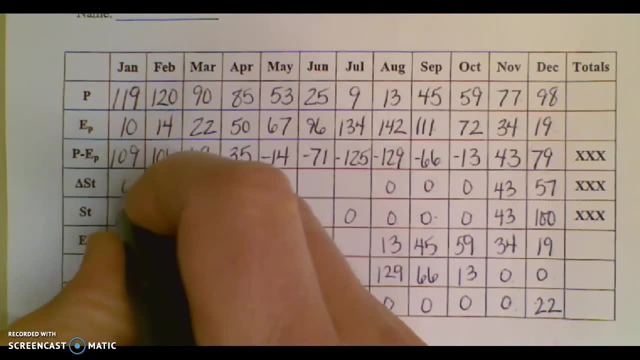 Definitely have more than enough water. So the 109,. the first thing you want to do is to try to put it in storage, But the previous month I already had a full storage, So my storage remains full, which means the change is zero. 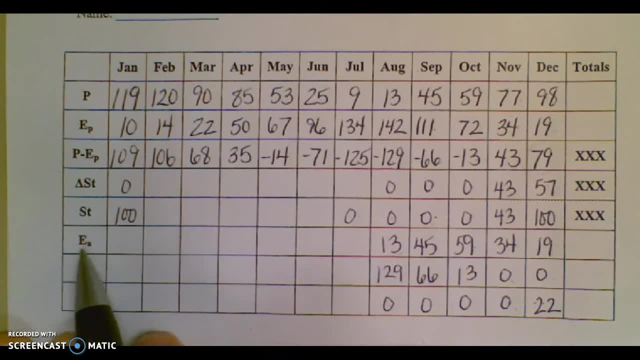 So none of this 109 went into storage. So I'm going to put it in storage. So I'm going to put it in storage. So we're going to put it in storage. So we're going to put it in storage. Actually, evaporation equals the potential. I had more than enough water. 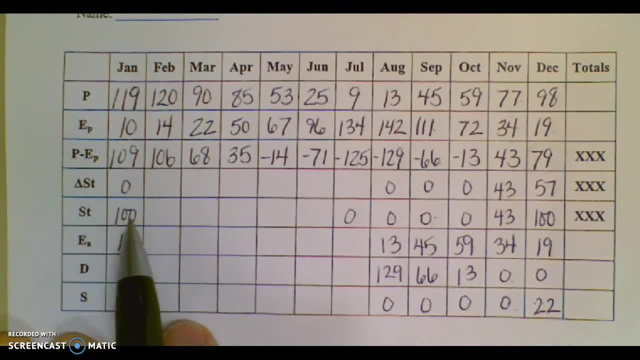 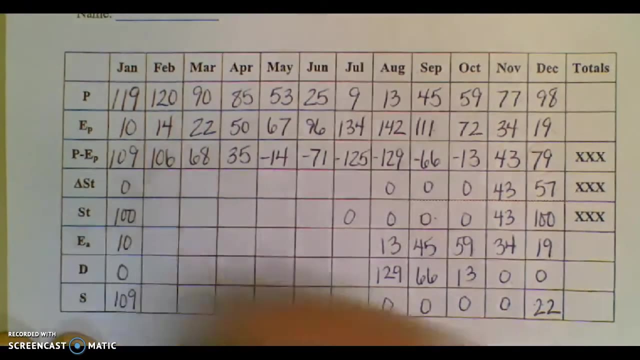 I'm not running a deficit. As long as you have water in storage, you can't run a deficit. Storage has to be down to zero before you can have a deficit. And my surplus? Well, since none of this extra 109 went into the ground, all of this 109 is my surplus Now. 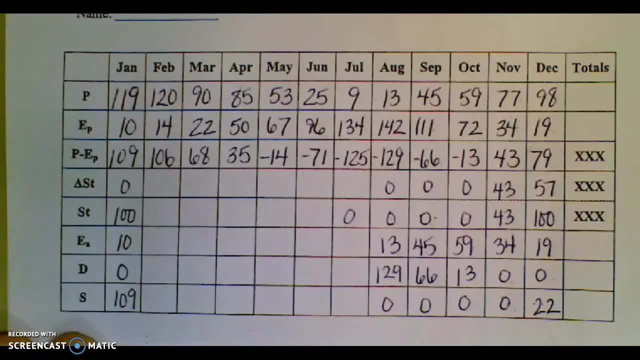 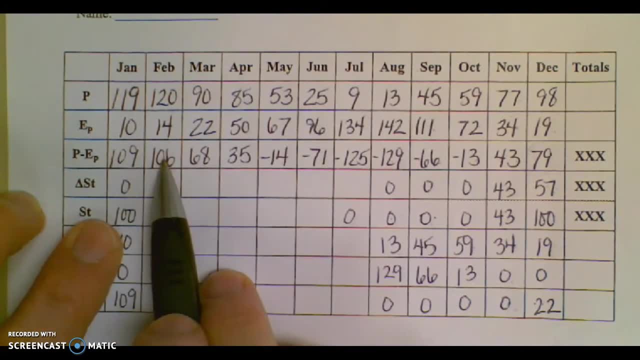 for the rest of this, I'm going to go ahead and put it in storage. I'm going to go horizontally, just to give you a sense of what it's like to do that. So my storage it's full. I'm trying to put more water in but I can't, So this stays. 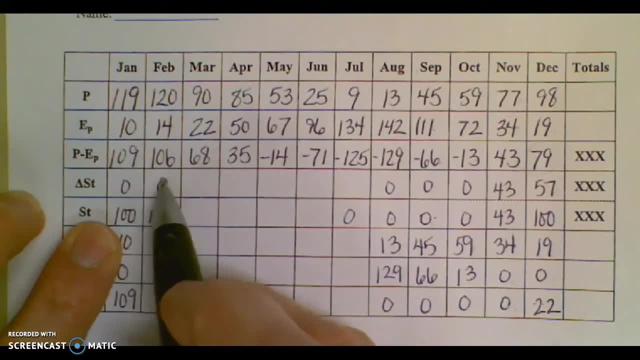 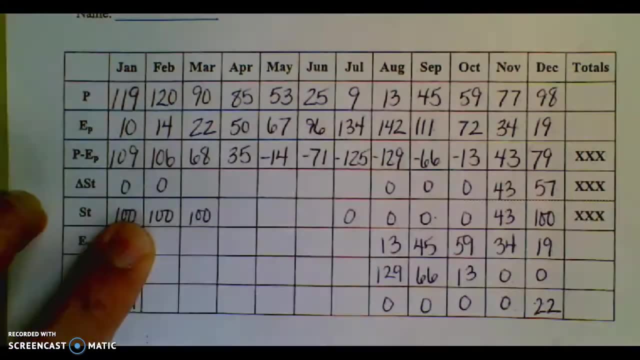 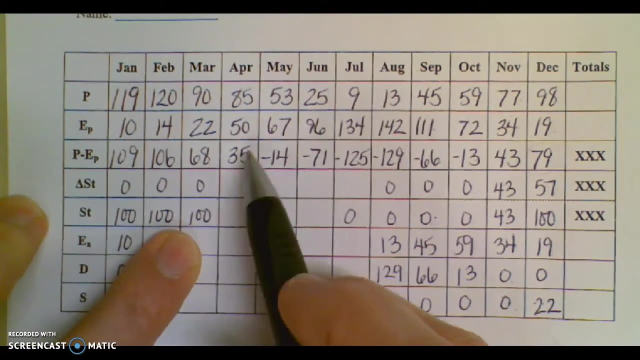 at 100, which means the change is zero. right, 100 plus zero is 100.. Still have extra water in March Trying to put it in storage, but I can't. Stays at 100.. The change is zero, Trying to put the 35 extra millimeters of water that fell from the sky. 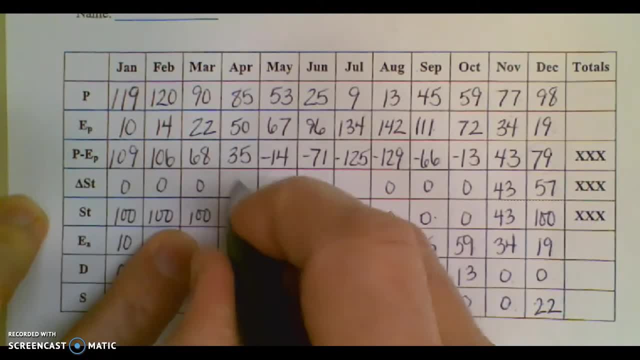 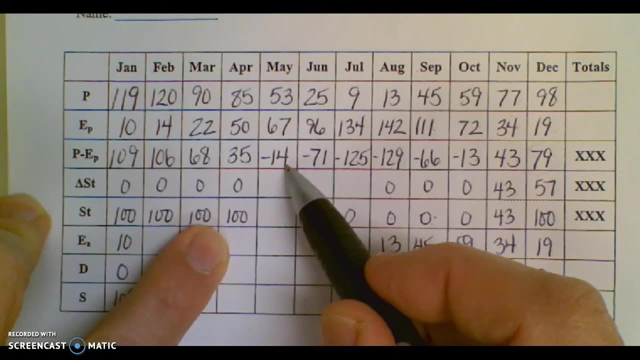 in April into storage. still can't 100, zero In May. it looks like I'm short. Where do you go to get the extra water? I go into storage, So I'm going to tap into that. How much am I going to take out? Well, I'm short- 14,. so 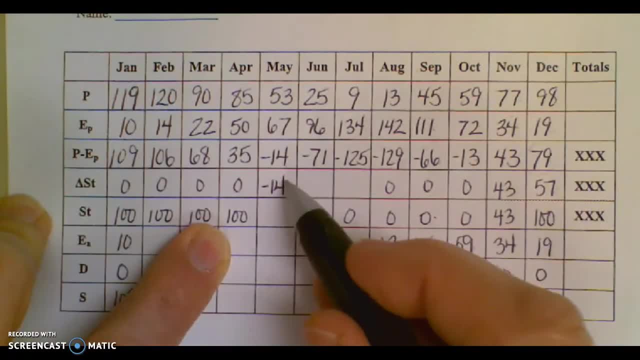 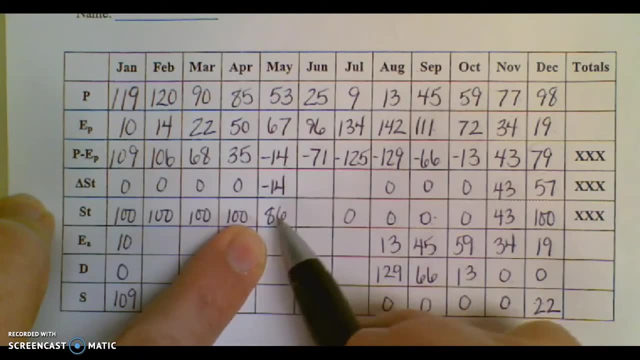 let's take the 14 out. 100 minus 14 is 86.. The next month I'm short, 71.. Do I have enough in storage? Yes, I do. I've got more than 71 in storage, so let me take. 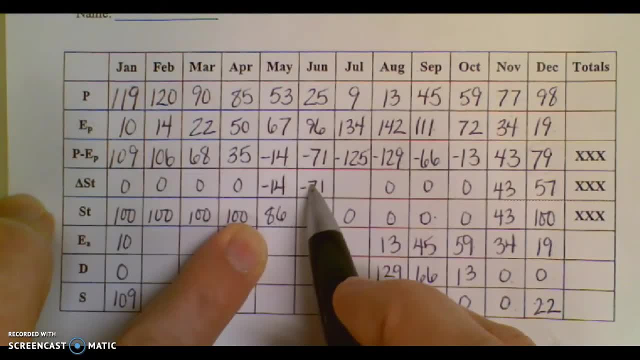 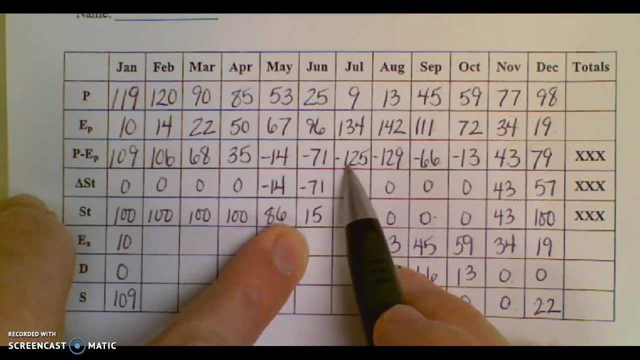 all 71 out. 86 minus the 71 leaves me with 15 millimeters in storage, And for the month of July I wanted 125, but I only have 15 in storage. So I'm not going to get to my 125, but I can at least get the 15 out. 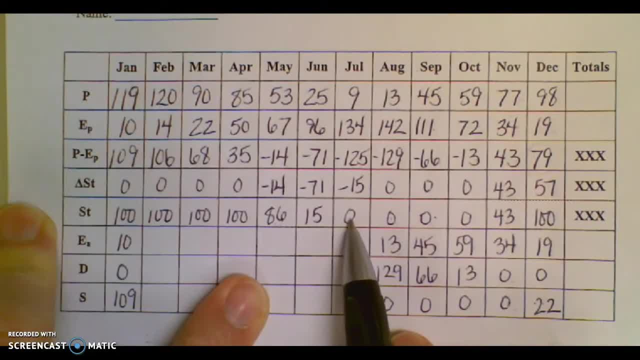 So I'm going to take out the 15, and that brings me back to where I started, from a storage of zero. Now let me go through here your actual evaporation. I want it to evaporate 14 as long as I have. 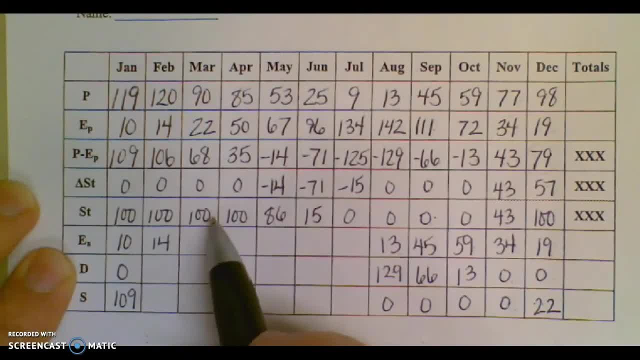 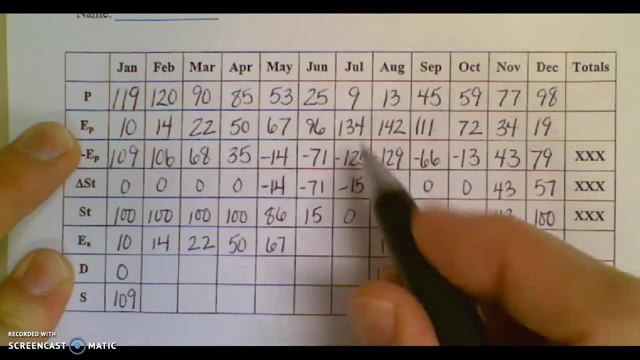 water in storage. That'll be the same. Same thing for March: There's water in storage. It's the same. April: I have water in storage. I can copy that down. Same thing for May 67.. And then June: I still have water in storage. I'm using water. 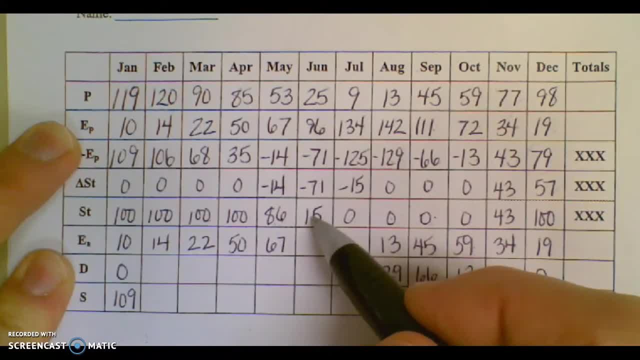 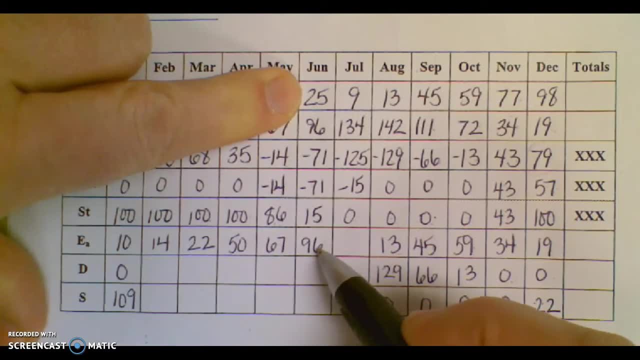 That I didn't get from the sky. I'm using the water from the ground, but I'm still able to make that up. So if I look at my 96 that actually evaporated, only 25 of that 96 came from the sky. The 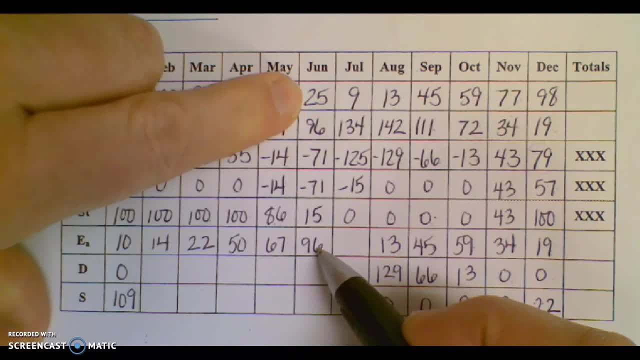 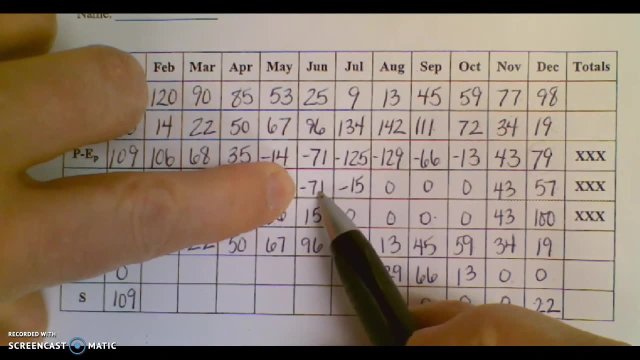 other 71 came from the ground, But a combination of the 25 and the 71 I took out of the ground that equals my 96. Don't let this negative sign fool you. You're not subtracting 71.. Well, you are from the. 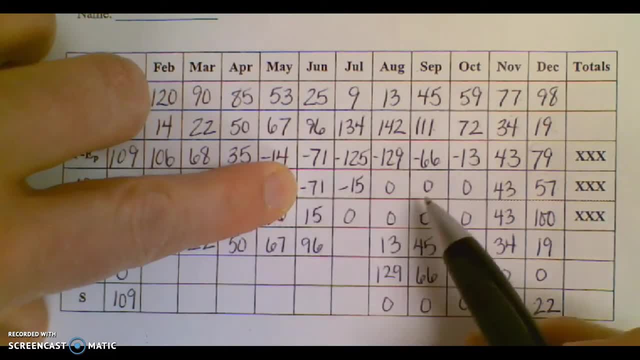 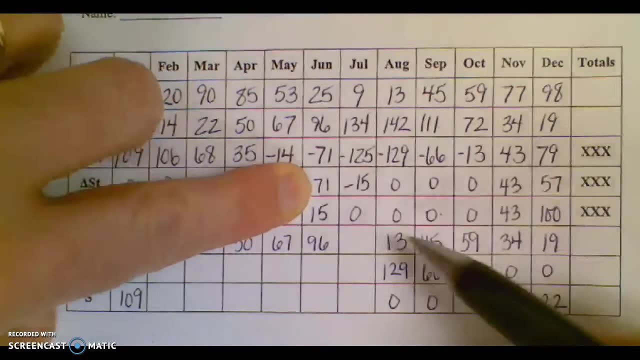 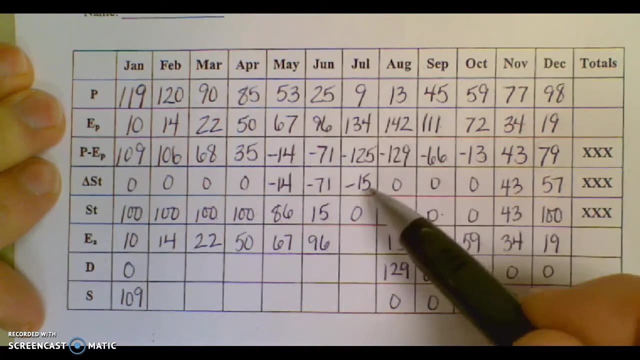 ground, but really the negative sign just tells you you're taking it out of the ground. Really, It's 71 millimeters. It's 71 millimeters of water added to the 25 to get you the 96.. So what about July? What did I do for July? I evaporated the 9 plus the 15.. Well, 9 plus. 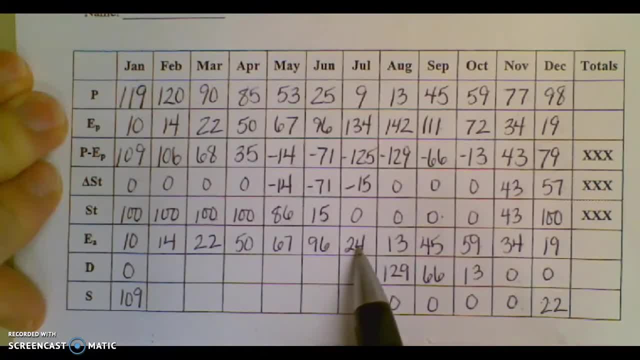 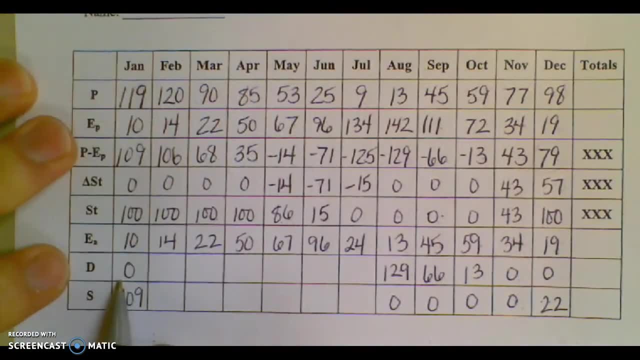 15 is only 24.. That's how much evaporated. I didn't have any more water than the 9 that fell from the sky and the 15 that came out of the ground. Deficits, No deficits, as long as I have storage. 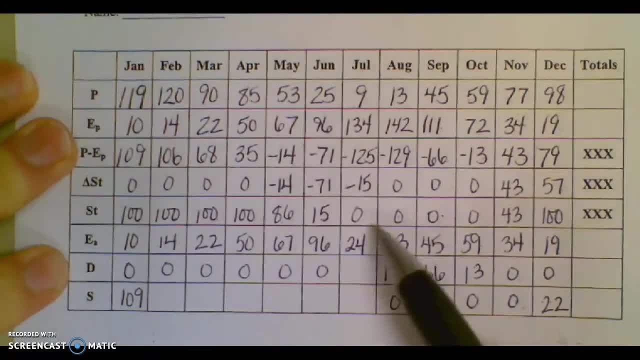 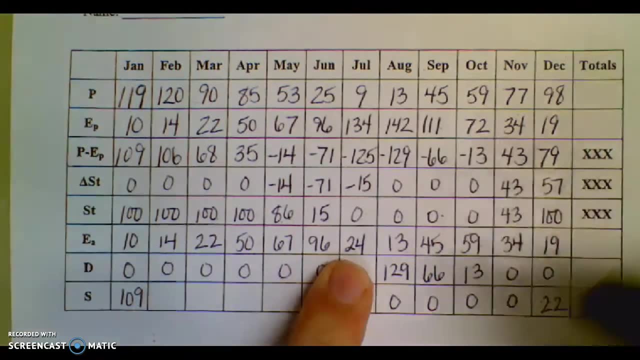 So 0, 0, 0, 0, 0.. 0.. I am running a deficit here. I wanted to evaporate 134, but I only evaporated 24.. So it looks like I'm short 110.. 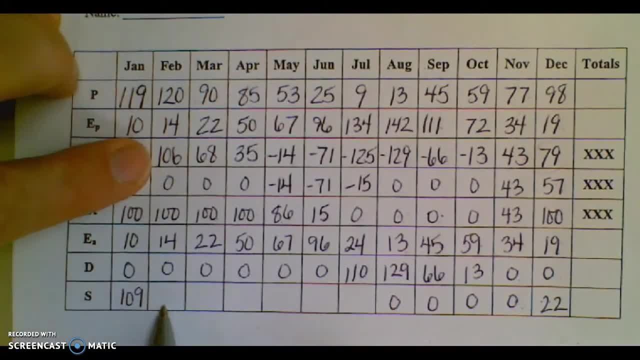 Surpluses, Surpluses. here It looks like I've got 106 extra millimeters of water. None of that extra went on the ground. Looks like I've got 68 extra millimeters for the month of April, Right, 90 minus the 22. 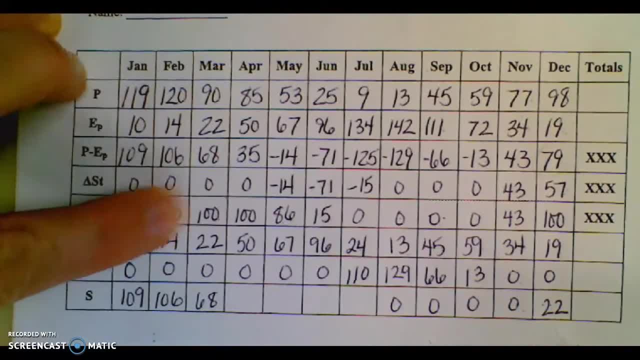 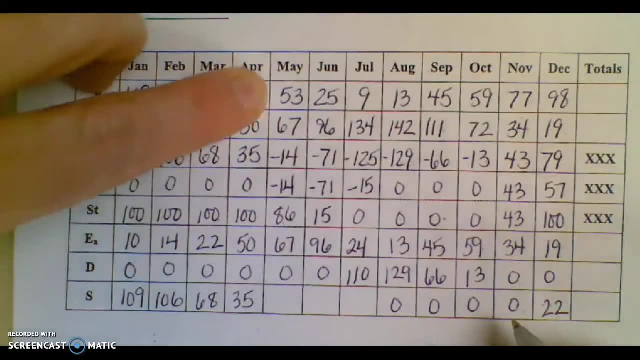 that wants to evaporate is going to be 68. None of that 68 goes on the ground, so it all is surplus. Same thing happens in April. I've got a surplus of 35.. In May- notice- my storage went down to 86.. You can't have a surplus unless your storage. 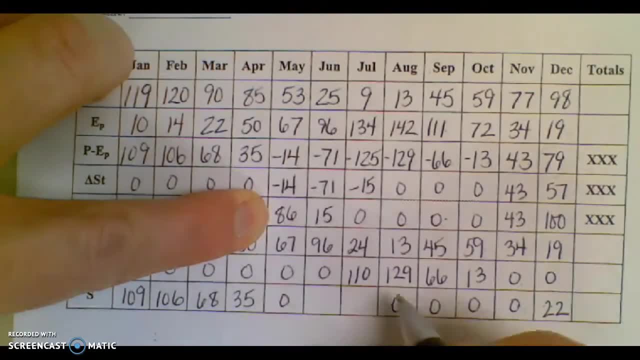 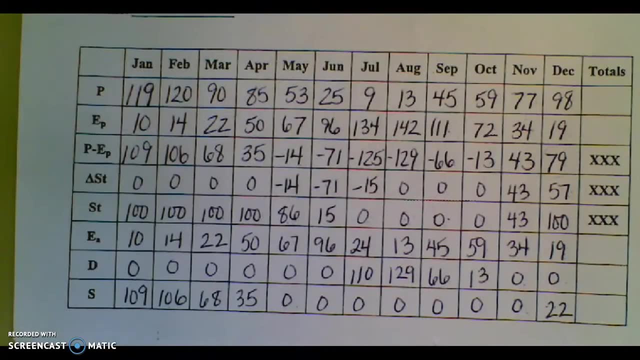 is totally full. It is not. It's not 100.. So no surplus, no surplus and no surplus for these months. My storage is not 100.. Again, You can do it horizontally, You can do it vertically, It's your choice, Whatever you're. 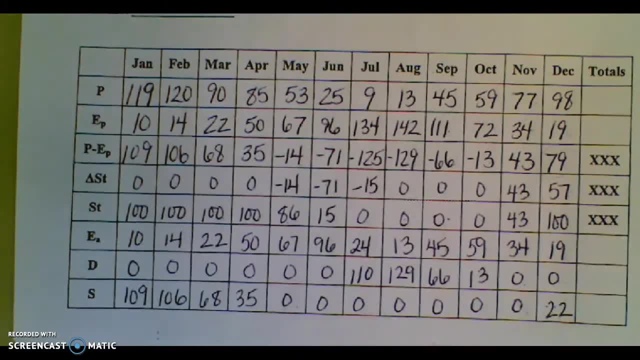 more comfortable with. I would encourage you to go through. Watch this video again. if you need to Pause it- I may have been speaking too fast- Feel free to rewind it. That's the great thing about the video: You have the control. I hope this helped. Have a good day.